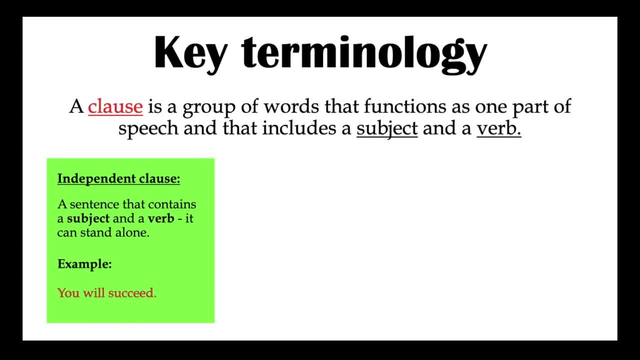 For example: you will succeed. You is the subject and succeed is the verb. This sentence makes sense on its own. therefore it's an independent clause, Dependent clause. This contains a subject and a verb, but it cannot stand alone. For example: 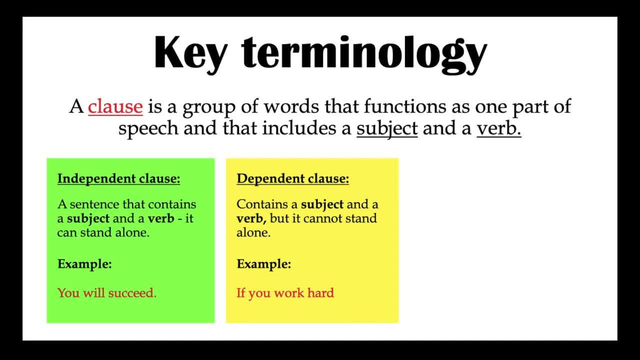 If you work hard, The subject is you and the verb is work. However, the sentence does not make sense on its own as it's incomplete. therefore, it's a dependent clause. It depends on something else in order for it to make sense. 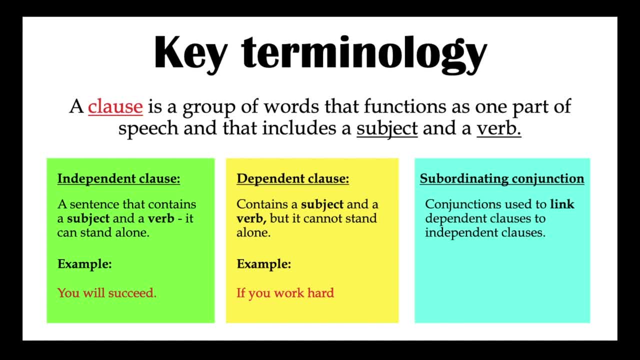 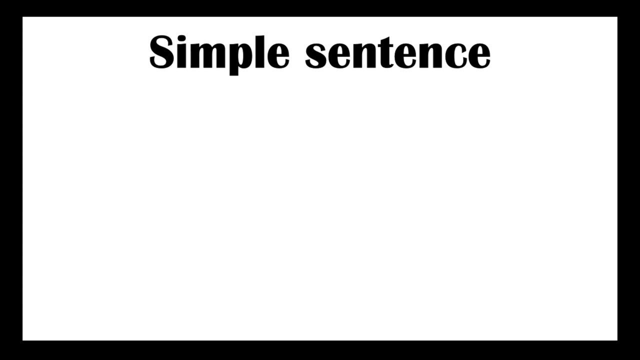 Subordinating conjunction. These are conjunctions used to link dependent clauses to independent clauses, For example: If you work hard, you will succeed. Now let's go through the four sentence structures: Simple sentence: A simple sentence contains at least one complete verb. 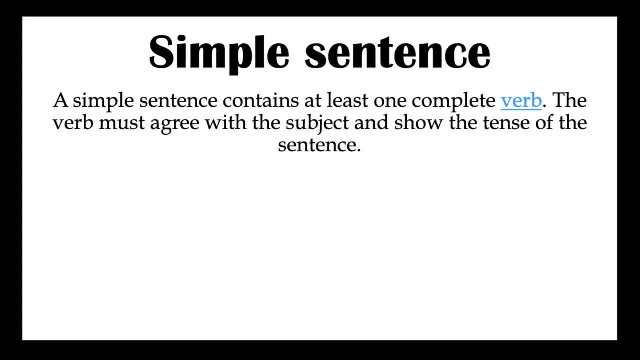 The verb must agree with the sentence, The first one is the subject and the last one is the tense of the sentence. Let's take a look at an example. Sally kicks the ball. Sally is the subject, Kicks is the verb And the tense used is the present tense. 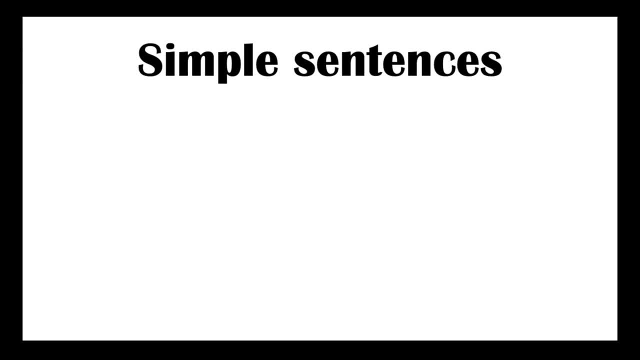 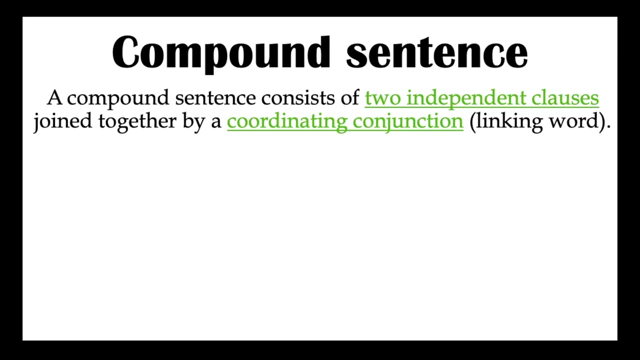 Let's take a look at some more examples of simple sentences. ben forgot his homework, tom kicked the ball. i ate lunch, emma waited for the train. compound sentence. a compound sentence consists of two independent clauses joined together by a coordinating conjunction. let's take a look at an example. he was hungry. this is an independent. 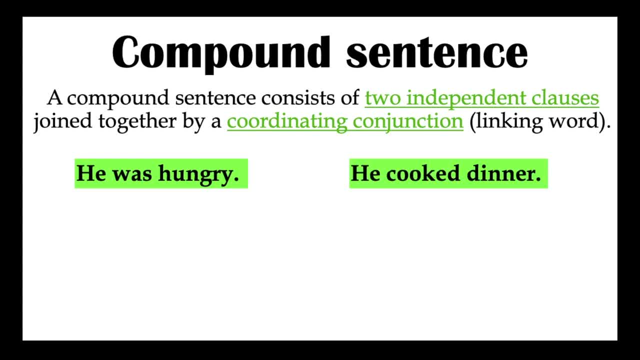 clause: he cooked dinner. this is also an independent clause. we can now join the two independent clauses by using a coordinating conjunction. using the coordinating conjunction so allows us to form the compound sentence: he was hungry, so he cooked dinner. other examples of coordinating conjunctions include for, and, nor, but or yet so. 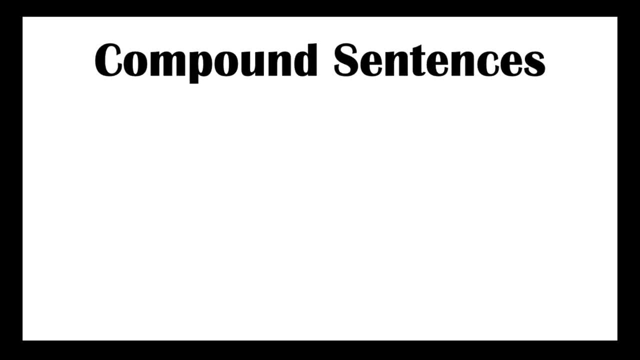 here are some more examples of compound sentences. i want to lose weight, so i must eat- eat healthy. she is rich, yet she is very humble. i'm hungry, but i don't know what to eat. complex sentence. a complex sentence contains an independent clause and a dependent clause. 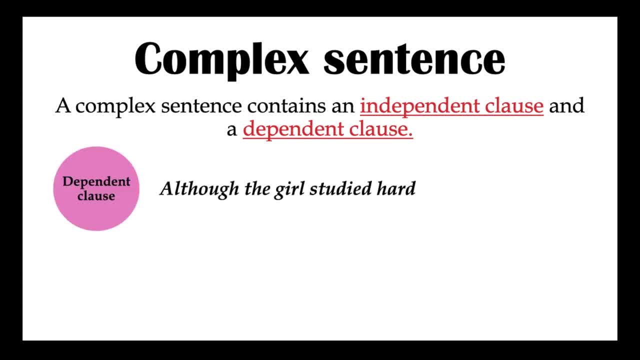 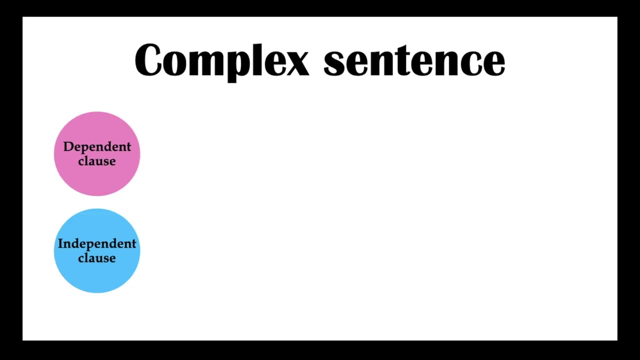 let's take a look at an example. although the girl studied hard, this is a dependent clause. it does not make sense on its own- she failed the exam. this is an independent clause. it does make sense on its own. we can join the two together to form a complex sentence. 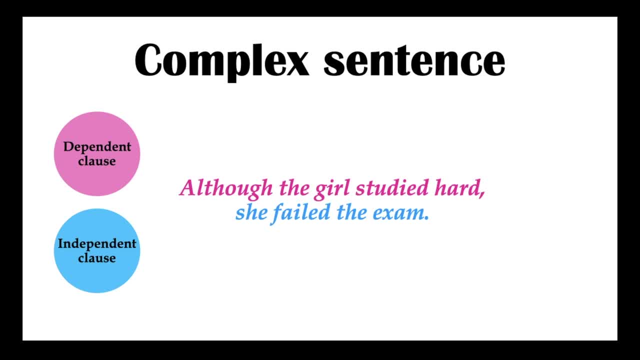 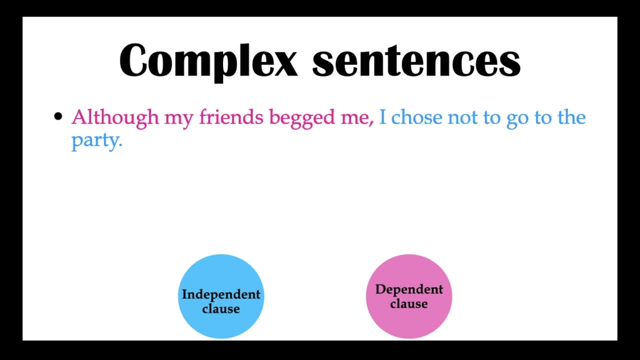 although the girl studied hard, she failed the exam. remember to add punctuation in the correct place when forming a complex sentence. here are some more examples of complex sentences. although my friends begged me, i chose not to go to the party. whenever prices are reduced, people buy more products. many people enjoyed the movie, however. 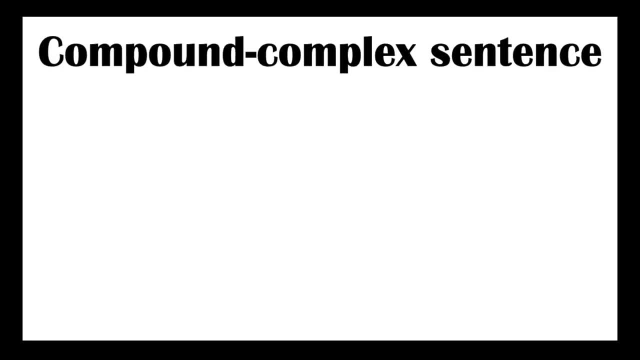 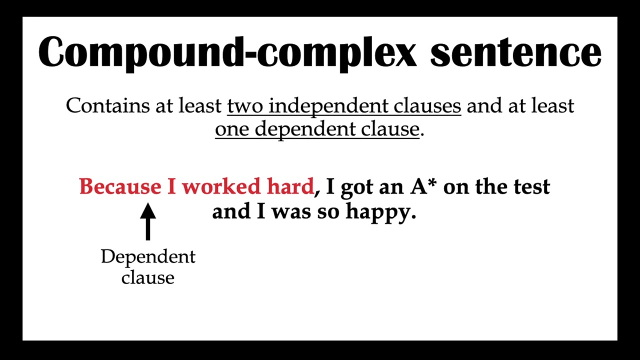 tim did not. compound complex sentence. a compound complex sentence contains at least two independent clauses and at least one dependent clause. for example, because i worked hard, i got an, a star on the test and i was so happy. this is the dependent clause. it does not make sense on its own.